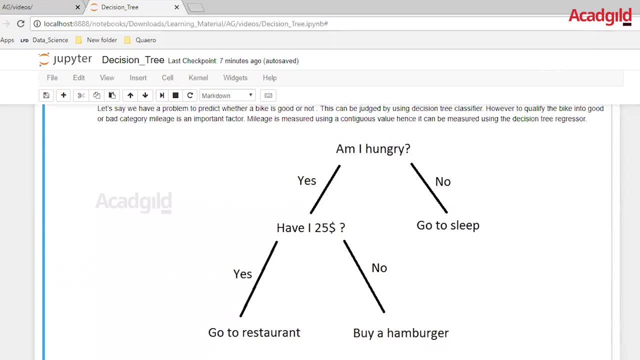 And if the answer is yes, then let us say I have a $25 note or not. If I have $25 with me, then I will go to a restaurant because I am hungry and I am not going to sleep and have something in the restaurant. 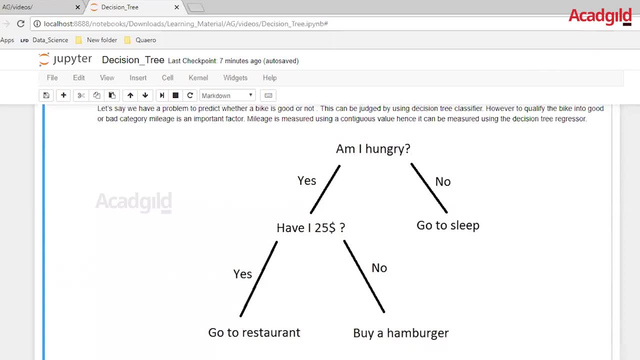 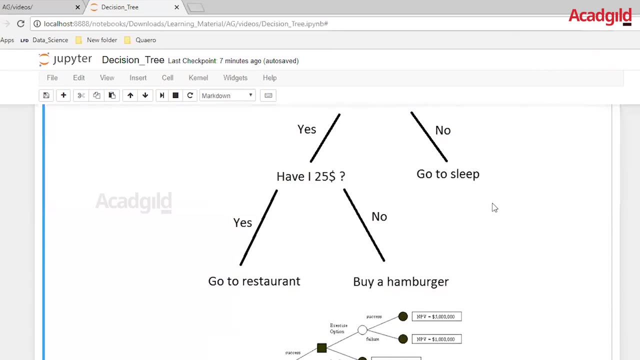 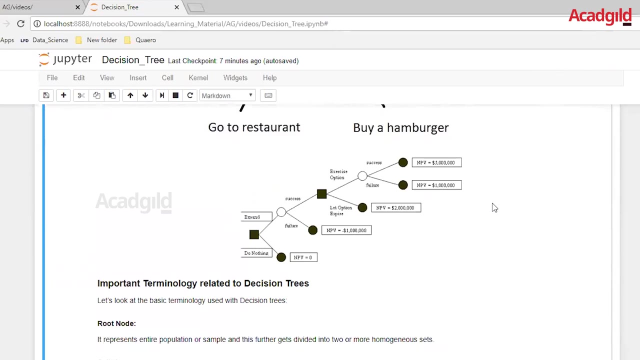 Otherwise I will buy a hamburger, which will be a cheaper option. So this is a perfect example for a classification problem using a dysentery. Let us try to look A regression problem using the dysentery. Say there is a stock in the market and we as a company are trying to figure out what. 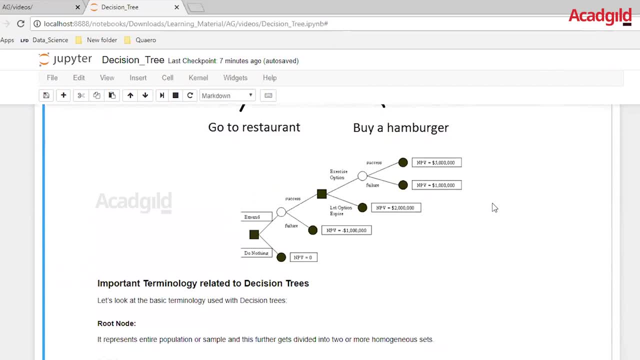 is the net present value of it. If, let us say, if the company is doing the expansion, then in that case there could be further two outcomes, which are success or failure, and if in case the company is not doing the expansion, then the net present value will be zero. 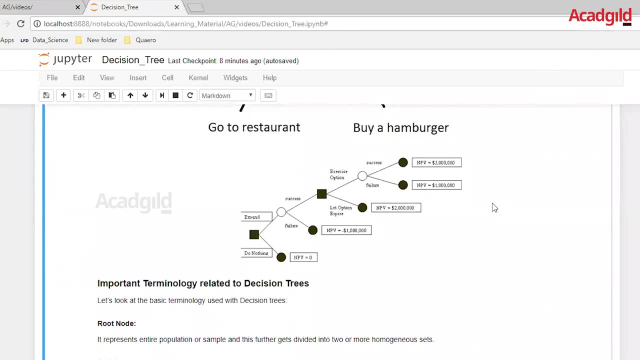 If the company is doing the expansion and there is a success, then we can exercise the option or we can let the option expire Again. This will result in two different scenarios in which there could be a success or there could be a failure. So, as we can see, there are different outputs corresponding to different scenarios. 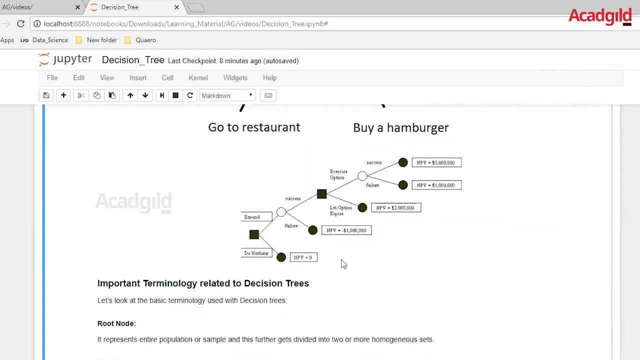 So what we are looking for is basically the different values which are coming for the net present value of the stock, And this is not a classic class label. this is something a continuous value. So this will come under the category of solving a regression problem using dysentery. 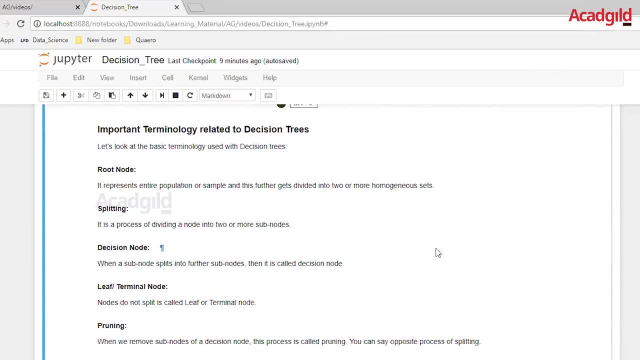 Let us go through few of the important terminologies which are related to dysentery. The first one is the root node. Root node represents the entire population or the sample, and it gets further divided into two or more homogeneous sets. By homogeneous sets we are trying to say that there are two sample of populations which 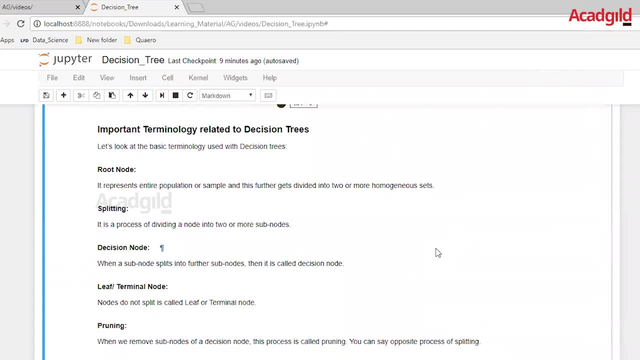 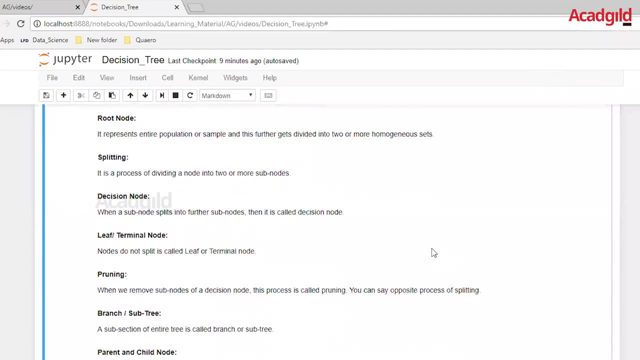 are same throughout. Next is splitting. Splitting is a process to divide any node into two or more sub nodes. It could be a root node or it could be a child node. The next is descent nodes. When a sub node splits into four sub nodes, it is divided into two sub nodes. 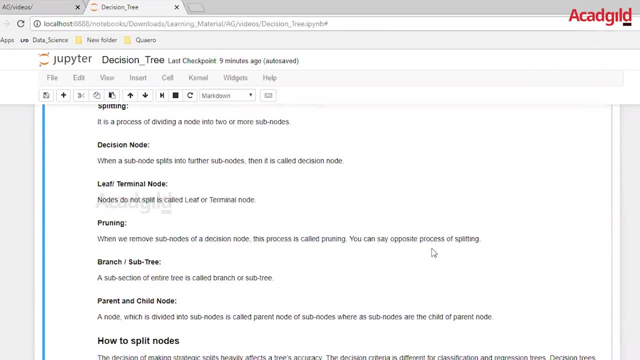 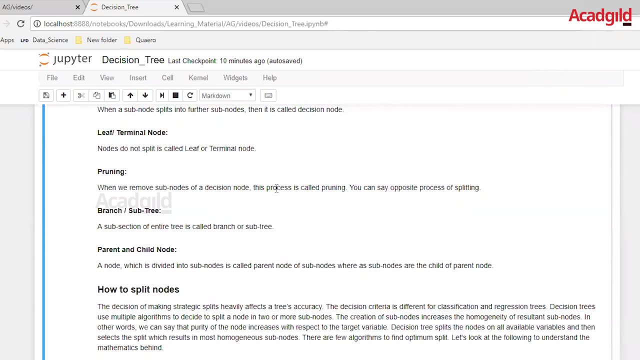 The next is descent nodes. When a sub node splits into further sub nodes, then it is called as a descent node. Using the different attributes in that given dataset, a descent or a split is taken on the descent nodes. Next is leaf or terminal node. 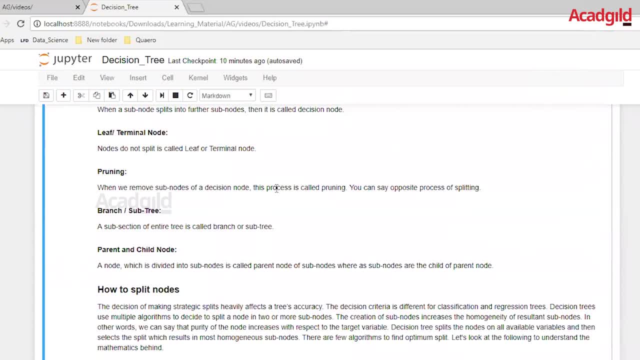 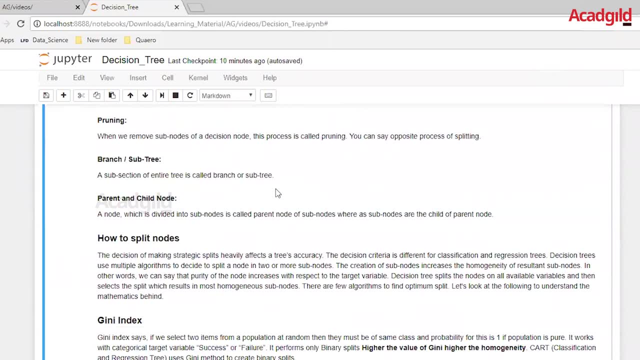 Leaf or terminal nodes are the final nodes of a tree and these nodes do not split further. Pruning: When we remove sub nodes of a descent node, this process is called pruning. One can say that the pruning process is an opposite of the splitting processes. 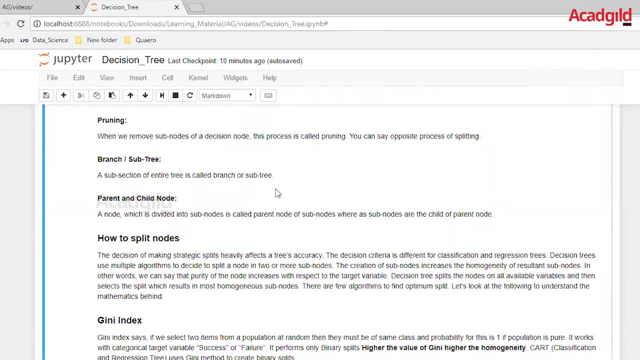 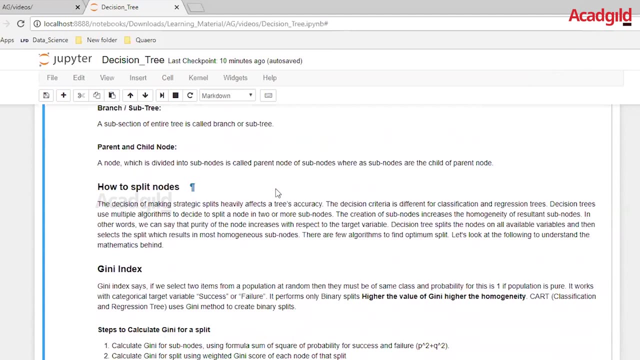 It is similar to the pruning done to the accuracy run to the actual trees. branch or subtree. A subsection of the entire tree is called a branch or subtree. A subtree could have a collection of nodes and branches. Parent and child node: A node which is divided into subnodes is called a parent node of subnodes. 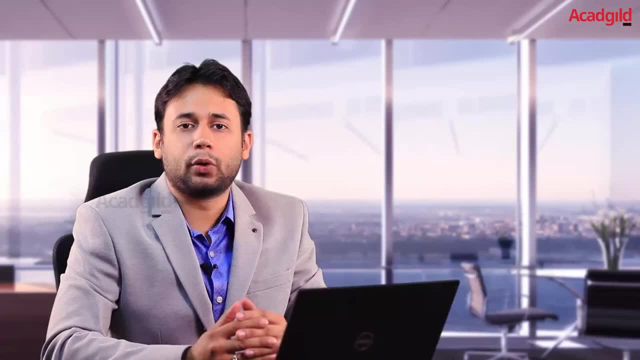 whereas subnodes are the child of a parent node. After going through the theory of the descent trees and few of the terminologies related to it, let's go through how to make a split in a descent tree. The descent of making strategic splits in a descent tree heavily affects its accuracy. 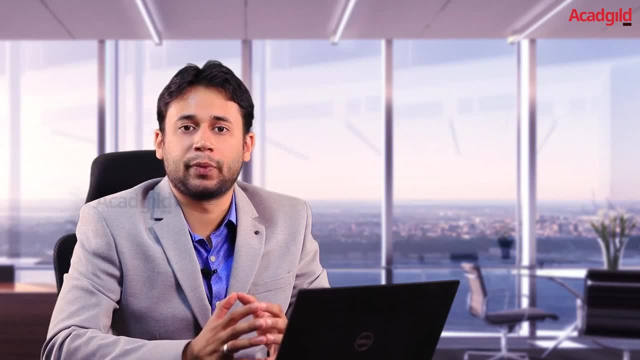 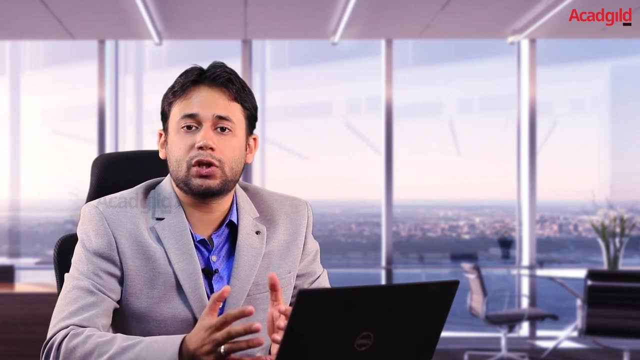 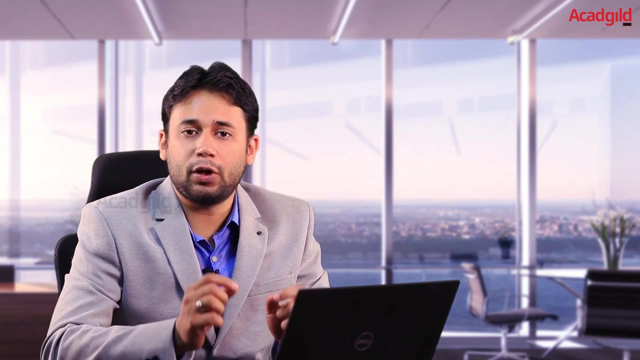 The descent criteria is different for classification and regression trees. Descent trees uses multiple types of algorithms to decide to split a node into two or more subnodes, and the creation of the subnodes increases the homogeneity of the resultant subnodes. In other words, one can say that the purity 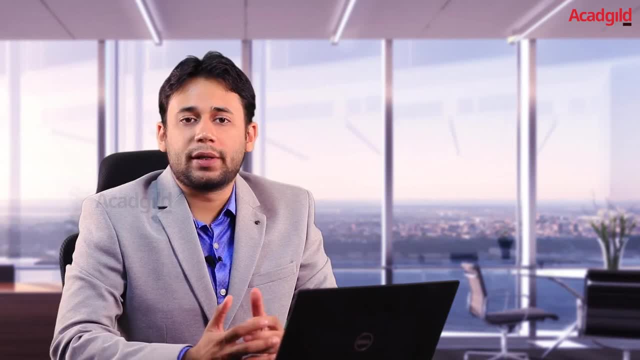 of the node increases with respect to the target variable. A. descent tree splits the nodes on all available variables in the given dataset. And. the descent tree splits the nodes on all available variables in the given dataset. And the descent tree splits the nodes on all available variables in the given dataset. 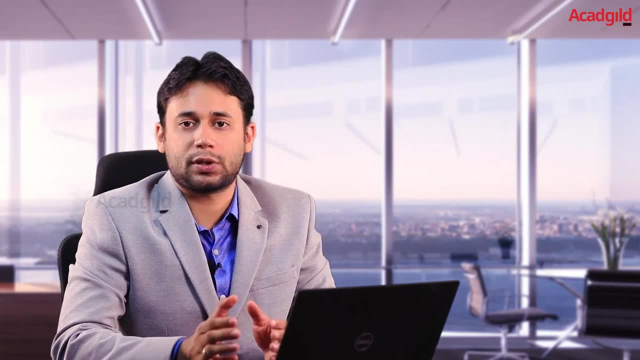 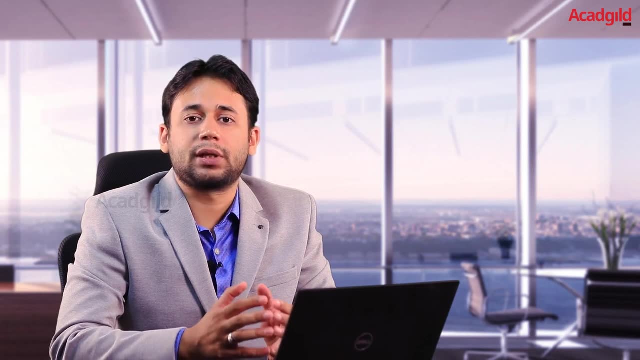 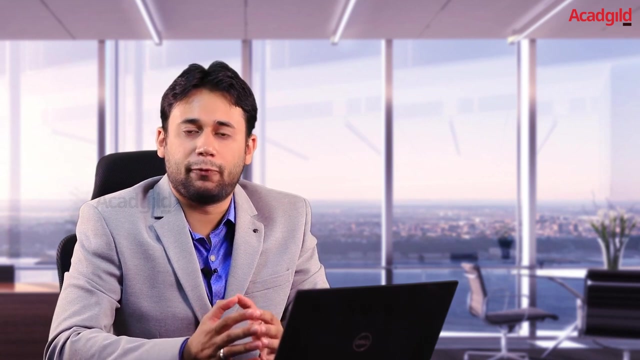 And then selects the split which results in the most homogeneous subnodes. There are few algorithms to find the optimum kind of split for a descent tree. Let's look at the following to understand the mathematics behind these algorithms. Let's go through the two criterion methods to decide the optimum split for a descent 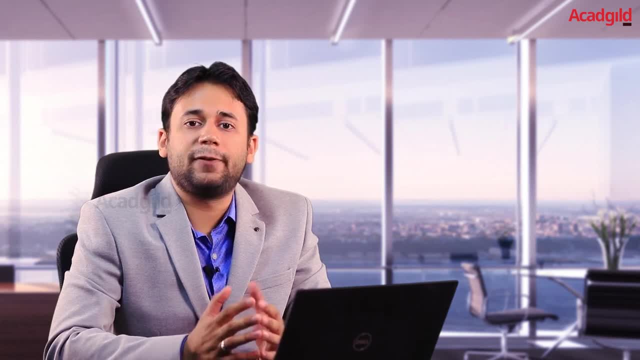 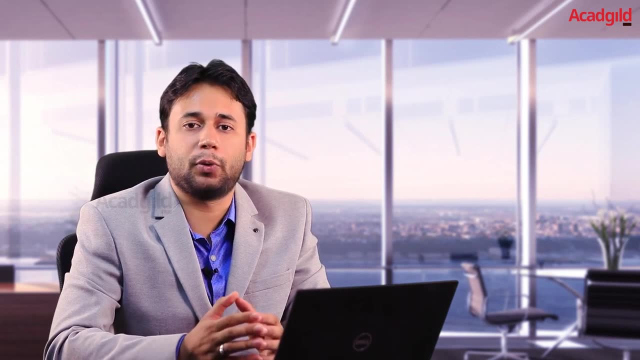 tree. The first of these is Gini index. In a Gini index, if we select two items from a population at random, then they must be of same class and the probability for this event is 1 if the population is pure, It works with categorical target variable: success or failure. 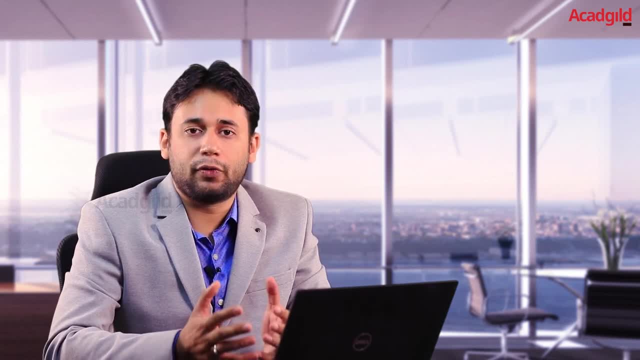 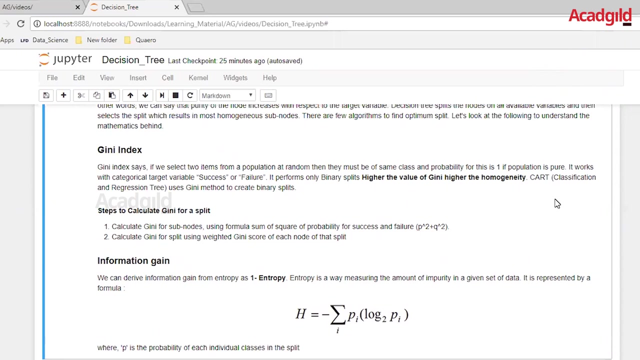 Gini index only performs binary splits. The higher the value of a Gini, the higher the homogeneity across the splits. CART, which refers to the classification and regression trees, uses Gini method to create binary splits. Let's go through the steps to calculate Gini for a split for a descent tree. 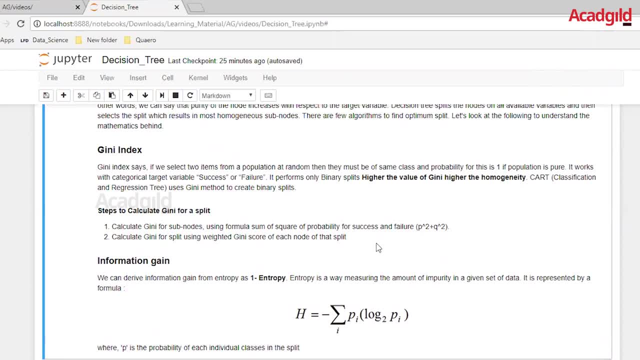 The first step is to calculate the Gini for subnodes using the formula of sum of square of probability for success and failure. Here P represents the probability for success and Q represents the probability for failure. The second step is to calculate the Gini for a split using the weighted Gini score of each. 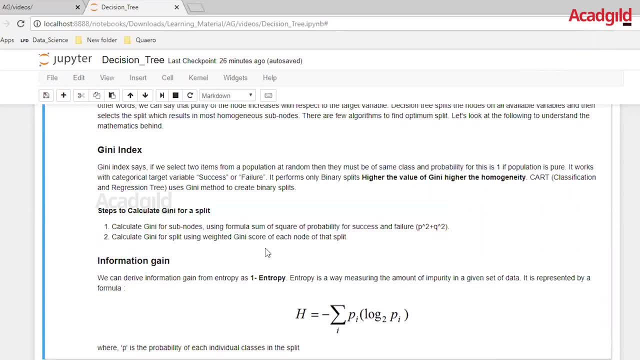 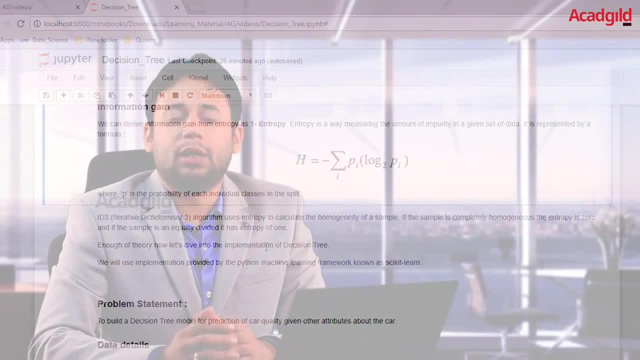 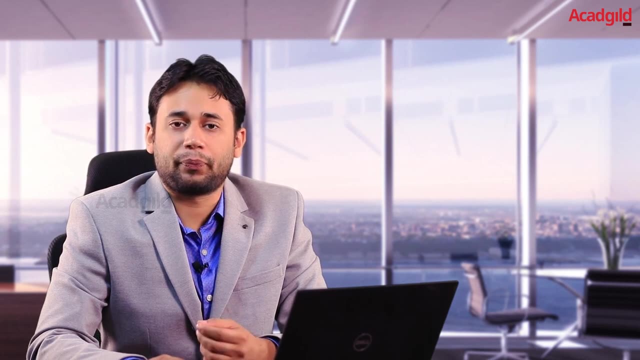 node of that split. The weights are given to the different attributes which are used to make the split, depending upon their relevance. Let's go through the second splitting criterion used for a descent tree. It is information gain. Information gain is calculated using the entropy. 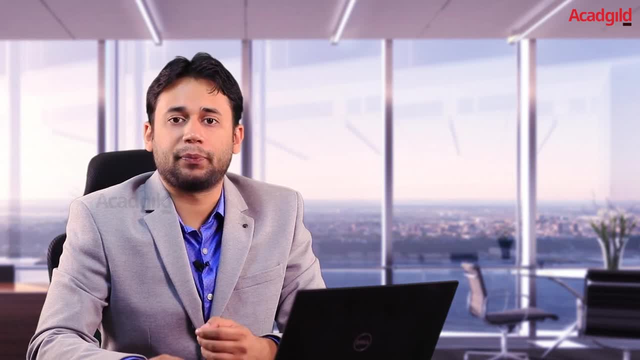 Entropy is a way to measure the amount of impurity in a given set of data. The iterative dichotomizer 3 algorithm is the predecessor of descent tree algorithm and it uses entropy to calculate the homogeneity of a sample. If the sample is completely homogeneous, the entropy is 0, and if the sample is unequally. 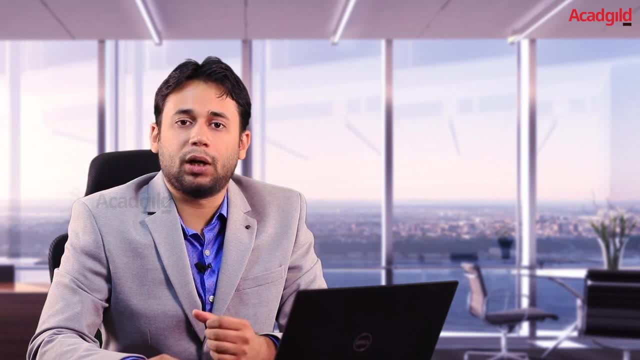 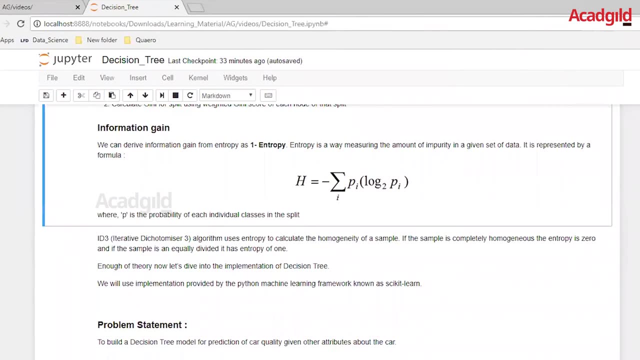 divided, it has entropy of 1.. Let's go through the formula for entropy. The formula for entropy contains the probability for each of the individual classes in the given split of the nodes, And it is determined by the probability for each of the individual classes in the given 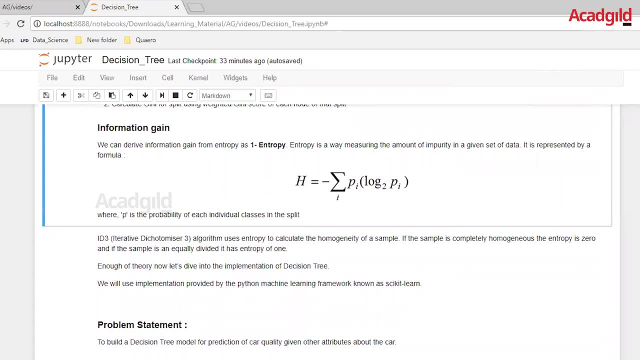 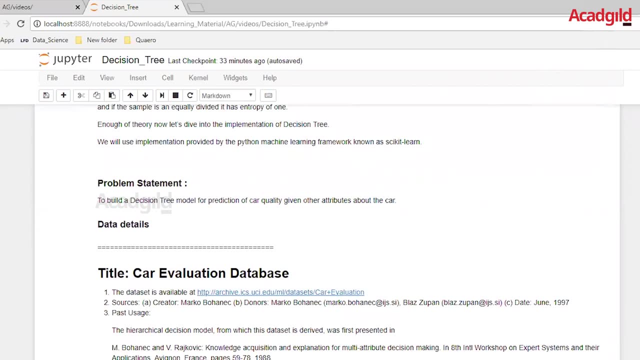 split, And it is calculated using the summation of the probabilities multiplied by the log of the probabilities. Enough of the theory, now let's go into the implementation. part of the descent tree. We'll use the implementation provided by the Python machine learning framework, which. 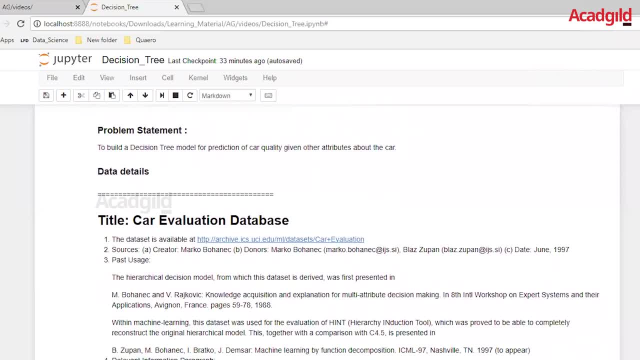 is scikit-learn library. The problem statement which we are trying to solve over here is to build a descent tree to predict the car quality, given the different other attributes of the car. The dataset which we have used is a public dataset. Let's go through the problem statement. 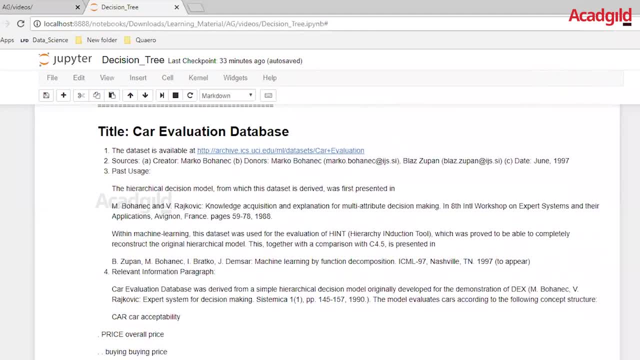 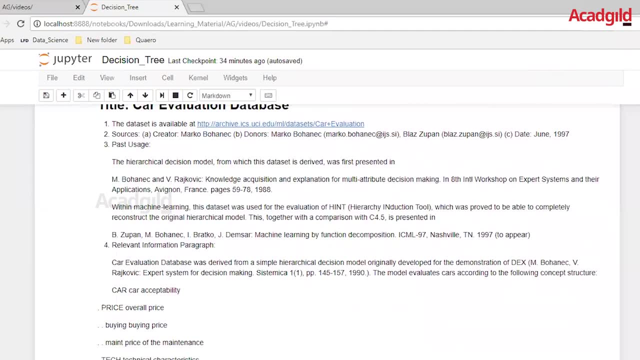 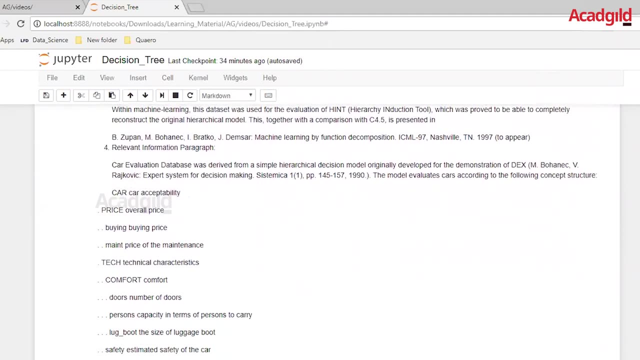 Let's go through the data details. The dataset which we are referring is a car evolution database and it is available on UCI depository. The dataset has been posted in 1997 and it features different characteristics of a car which are majorly the tech, comfort and price. 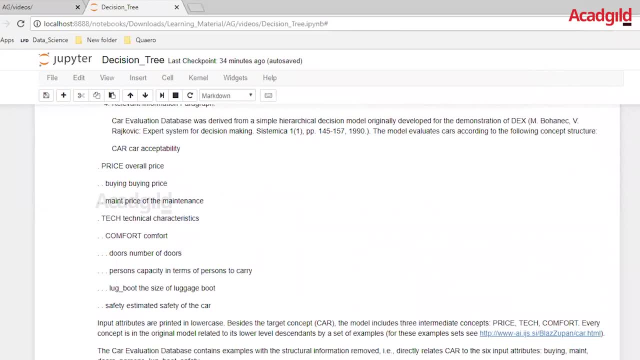 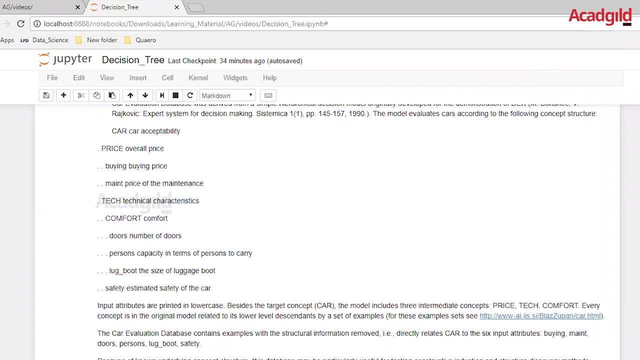 Regarding the price, we have the buying price and the maintenance price. Regarding the technical characteristics, we have the comfort features like number of doors, the capacity of the persons it can carry, the size of the luggage boot and the estimated safety of the car. 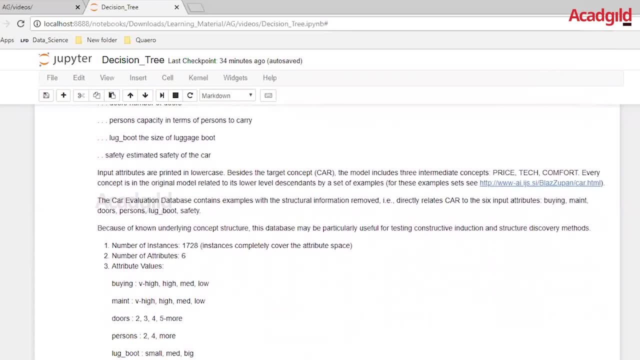 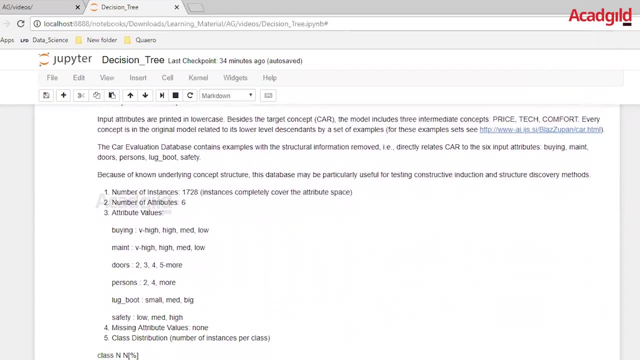 The final target variable which we have has got four different classes. which is? the car is acceptable, unacceptable, or it is a good or very good car. The total number of instances which we have in the given dataset is 1728 and the total number of columns or attributes which we have is 6.. 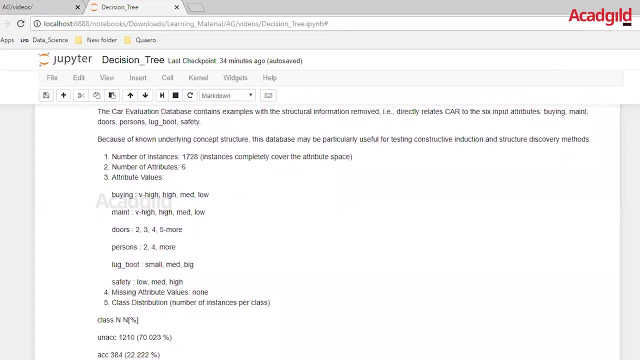 Considering the attributes, we have the different values. The total number of columns or attributes which we have is 6.. We have the different values which are majorly categorical, like the buying price, the maintenance price, the number of doors, the number of persons and the boot luggage, and also the 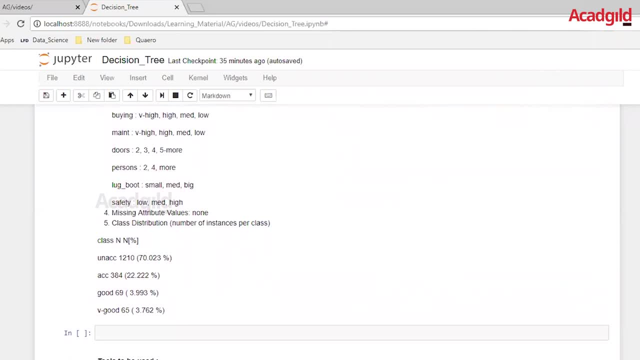 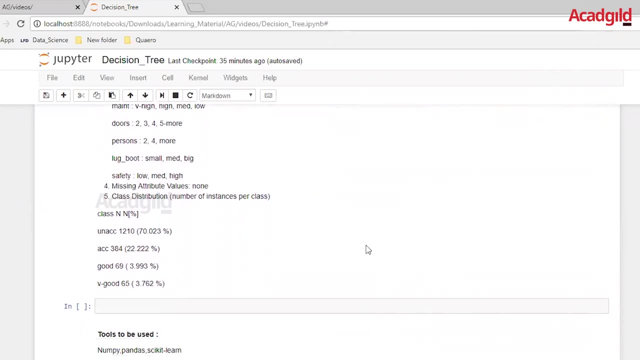 safety In the given dataset. luckily there are no missing attribute values and we are additionally given the distribution of the four different classes which are unacceptable, acceptable, good and very good. So we have a 70% for unacceptable, 22% for acceptable, almost 4% for good and 3.7% for. 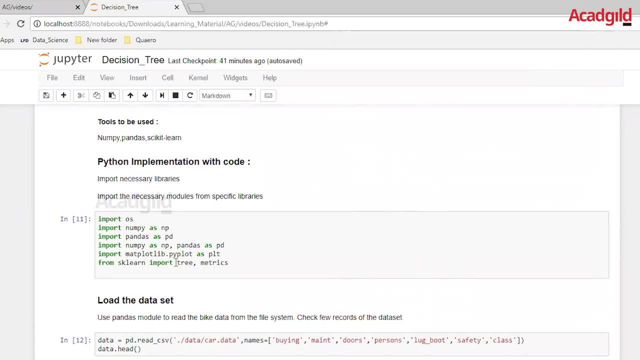 very good, Let's go with the Python implementation for a dysentry. Before I proceed further, I would like to request you to go through the Python tutorials from the Cadgill YouTube channel if you are a beginner in Python. Also, if you would like to refer, then you can go through the basic packages installation. 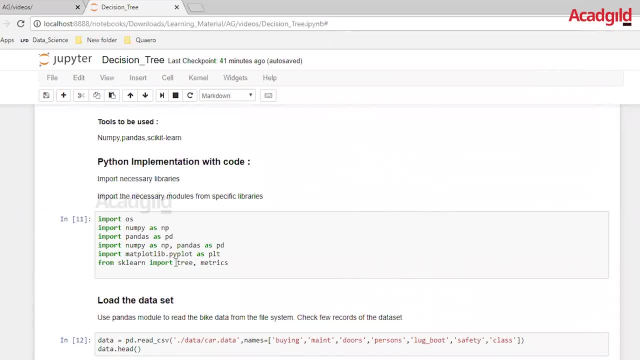 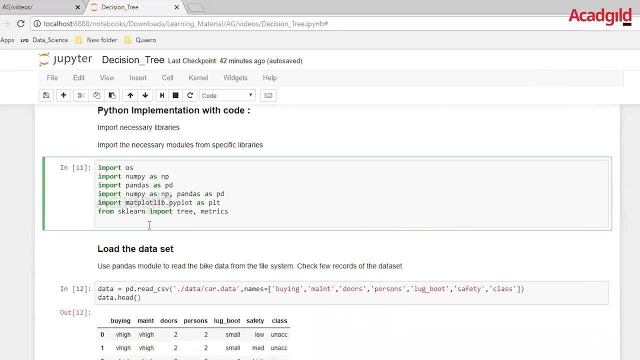 on the channel. We are going to use the libraries of numpy pandas- scikit-learn for this tutorial. Let's start with the implementation part. We are going to import numpy pandas- scikit-learn. From scikit-learn. we are importing two modules for tree and metrics. 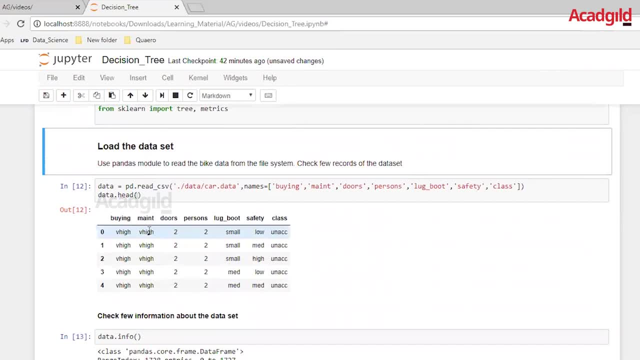 Let's start with loading the dataset. So I have downloaded the dataset from the mentioned URL above into a subfolder of data in the current working directory. The names which I am mentioning over here are the column names which are going to be present in the csv. 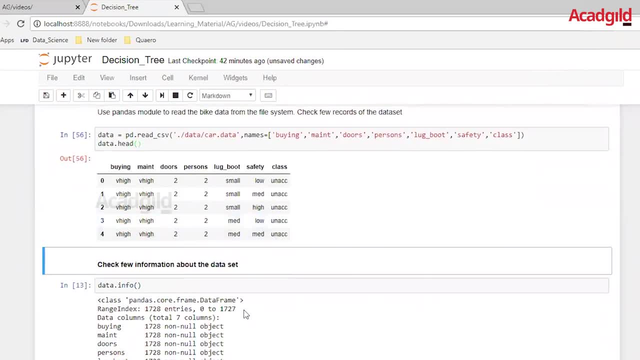 The datahead command will give us the view of the top five rows from the dataset. The datahead command will give us the view of the top five rows from the dataset. The datahead command will give us the view of the top five rows from the dataset. 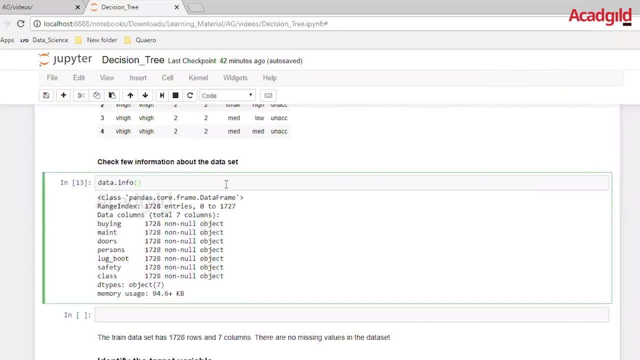 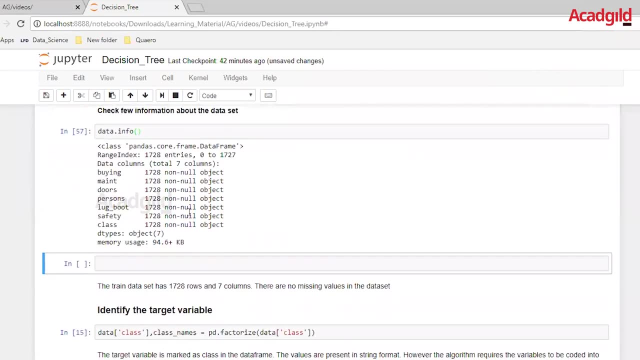 If you want to dig deeper more on the dataset regarding the type of the variables for each of the columns, then you can go with the datainfo command. It tells us there are 1728 entries, and then we have the six columns which are present. 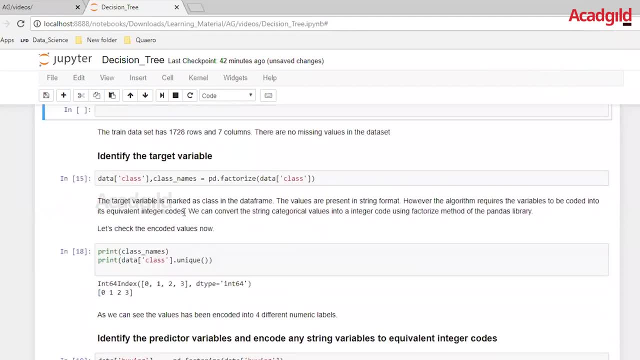 along with the class variable. Let's try to identify the target variable. The target variable is class, as we have already discussed during the dataset description, and it has got four columns. The target variable is class, as we have already discussed during the dataset description, and. 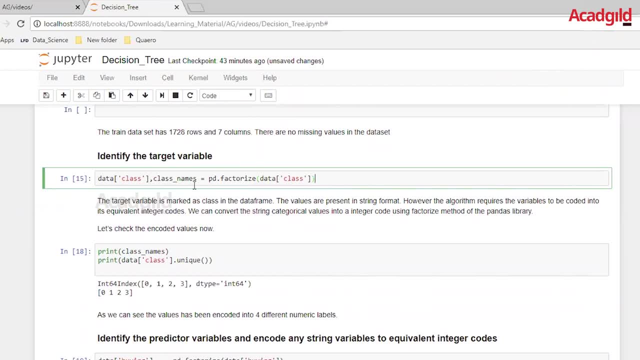 it has got four columns And it has four different classes, which is unacceptable, acceptable, good and very good. And it has four different classes, which is unacceptable, acceptable, good and very good. And it has four different classes, which is unacceptable, acceptable, good and very good. 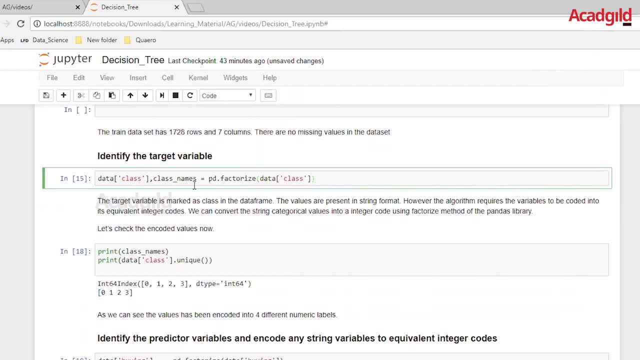 We are going to use the factorize command from panda library, which will help us to convert this target variable present in the string, to integer quotes. Let's execute this thing and see what is the output. As we can see, the class names are unacceptable. acceptable, very good and good. 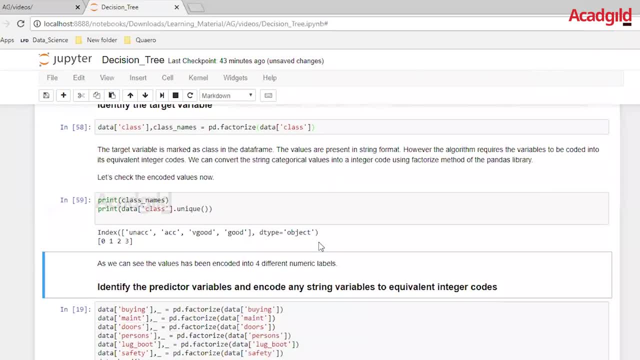 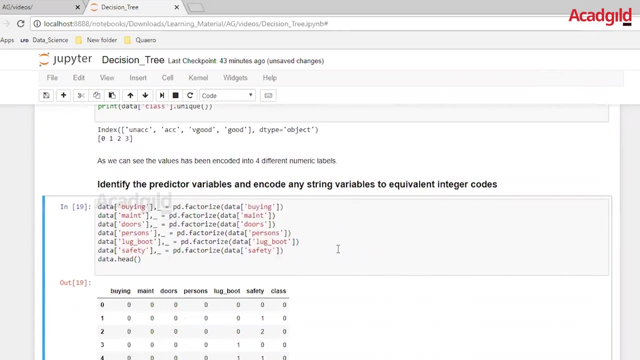 Corresponding to each of these class names. the data class column now contains 0,, 1,, 2, 3.. one-to-one mapping to the integer codes. We're going to follow the same exercise for the rest of the six columns, because all of the six columns in one or the 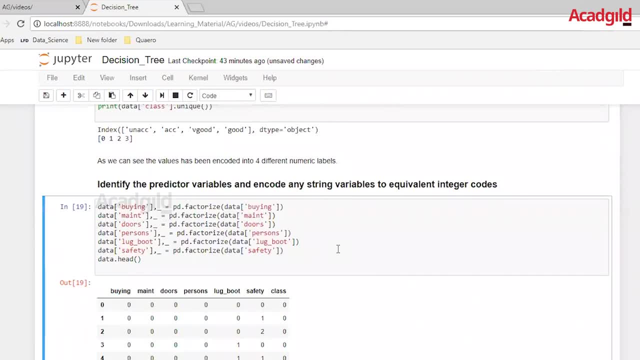 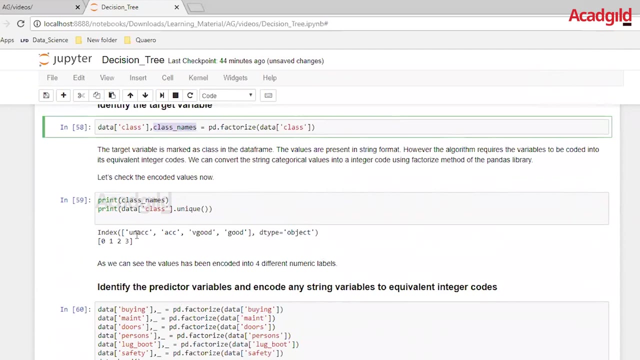 other way have string variables and we want to convert them to the factor columns or in a way in which we can get the direct integer codes. One more thing I want to mention over here. if you see the previous command in which we had the class names variable, the class names variables contains the strings original. 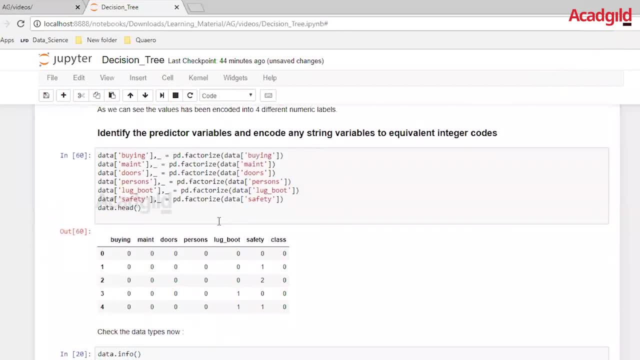 strings which are present in the given data set. While performing the same exercise for the rest of the six columns, we actually don't need these values to be printed, So we have just provided it with an underscore. so in this case, the function pdfactorize returns two values, so the second set of values will be lost. 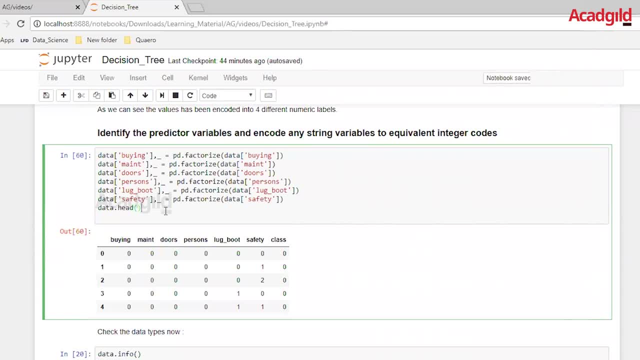 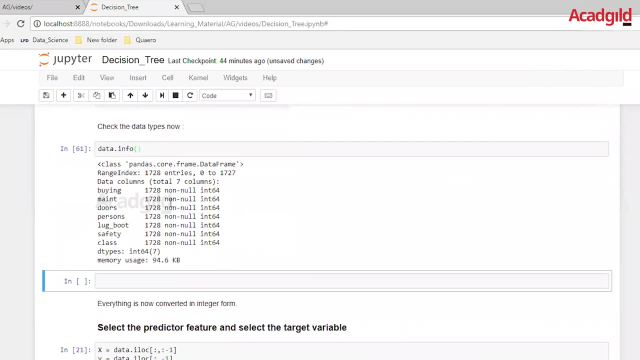 and we are just going to replace the columns by their integer codes. Let's turn the datainfo command again and then see how it has changed. So if you see the earlier it was object type for all of the seven columns and now it is converted to an integer type. So from now on, everything which is present in 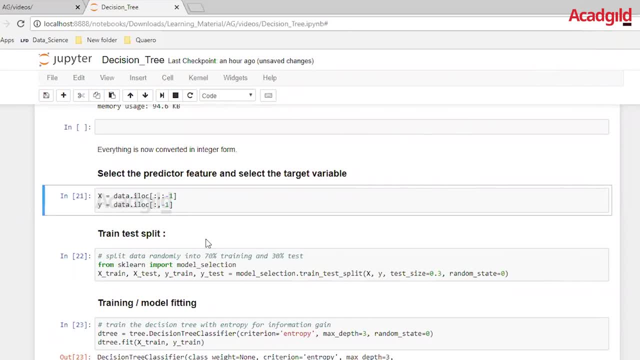 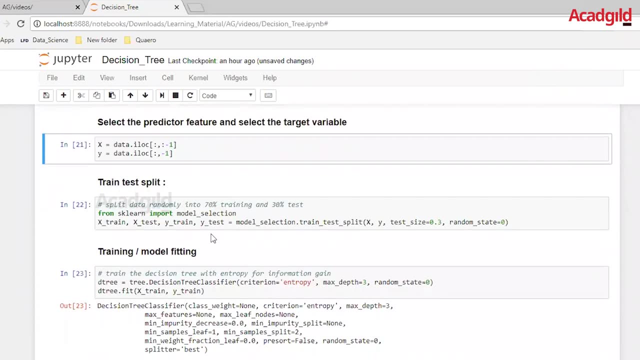 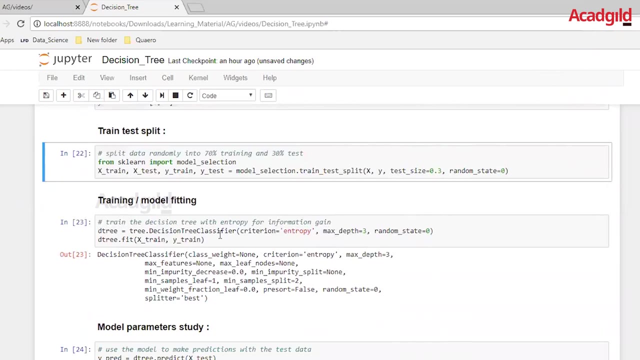 the data is of the integer form. Now we are going to divide the six features or columns into the x variable and the class variable as a y. The next step is to do a train test split, because we all know that in a supervised learning algorithm we are going to train our model on the train. 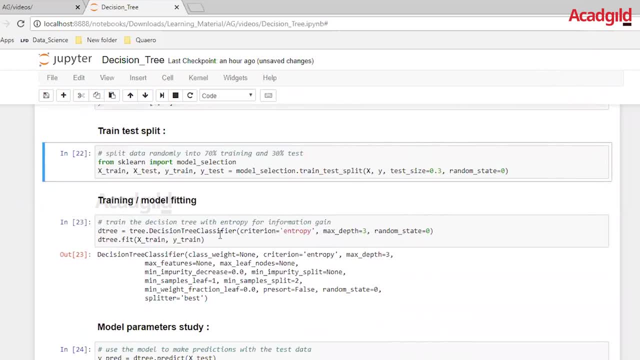 data set and when we are going to test and on the test data set. So we are taking a 70s to 30 ratio for the train and test data set For this. from the scikit-learn library we are importing the model selection module, The model. 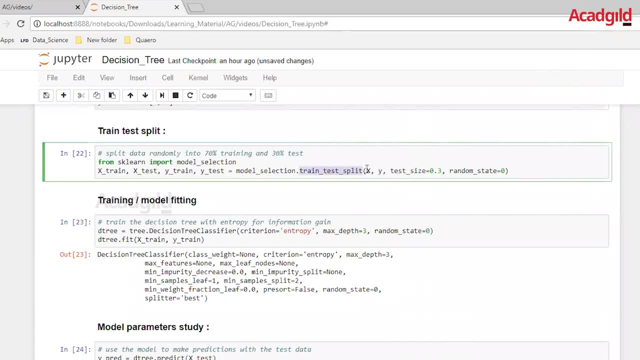 selection module offers a train and test split command which helps us to split both x and y variables into the given ratio of 70 and 30 percent. The random state variable is used to make sure that if someone else is reproducing the same problem then they are also having the same samples coming. 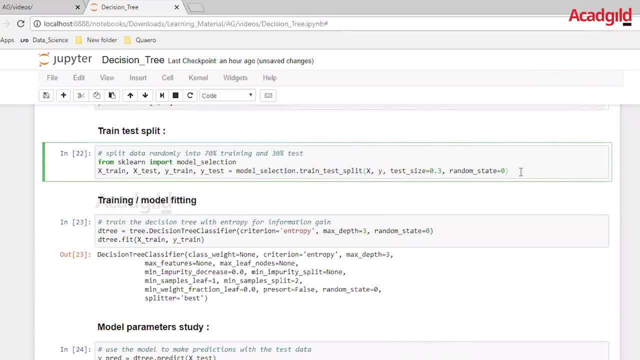 in the 70% of the train data set and same samples in the 30% of the test data set. This will make sure that, given the same data set for different users, they will have the same results. The next step which we have is to train or do the 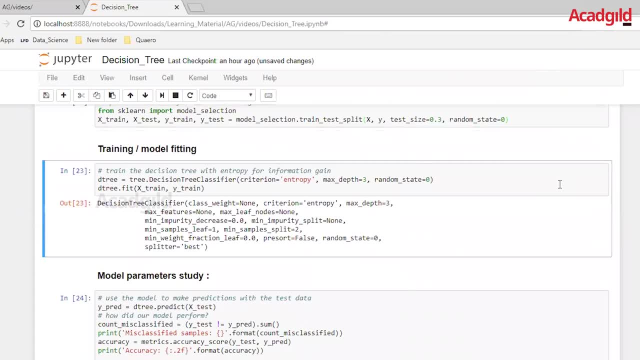 model fitting part. For this we are imported the tree module from the scikit-learn library, which internally contains the dysentery classifier. The criterion which we can use over here is either entropy, which is information gain, or the Gini. For the current exercise, we are using the entropy, We are specifying the. 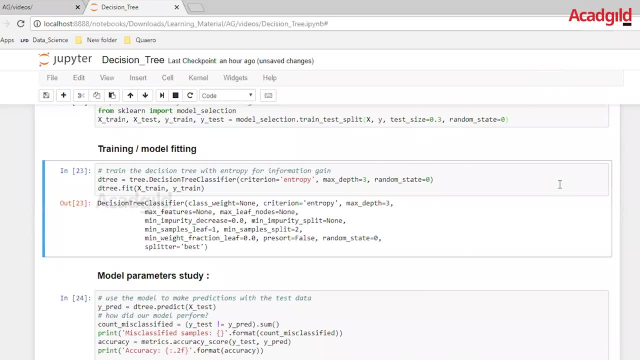 maximum depth of the dysentery as 3 and random state again as 0.. Internally, dysentery uses a lot of other variables as well which are chosen as a default. So like, if you can see in the output, we have the main sample split and the 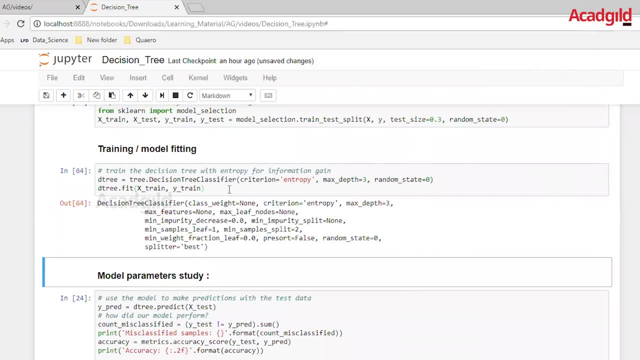 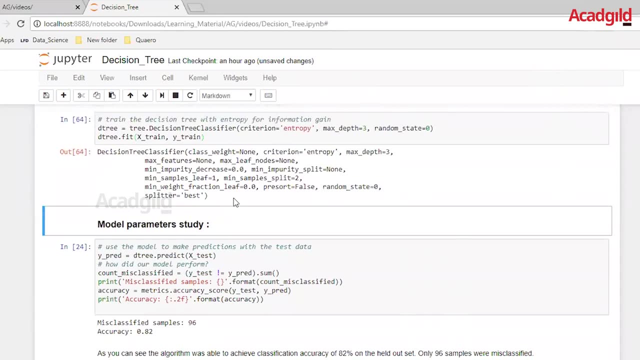 number of estimators and the number of variables. The number of variables is the maximum depth of the dysentery and the minimum sample sleep as well. So now we have got the dysentery object which has been fitted on the train, X variables and 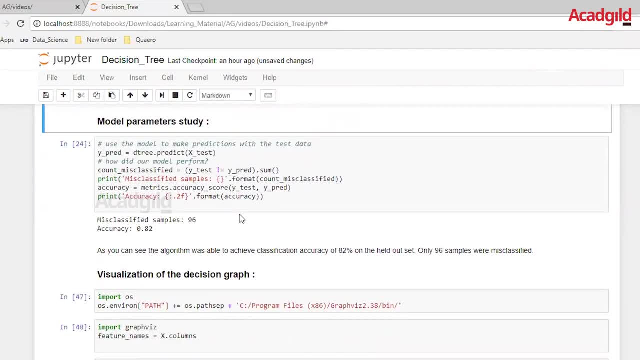 the train Y variables. The next step which we have to do is using this train model. we are going to predict it on the test data set- The test data set, which is the X test- and we are making a prediction corresponding to it and storing it under the variable 5 pred. This next step is followed by making a comparison between the actual data set and the sample sleep. 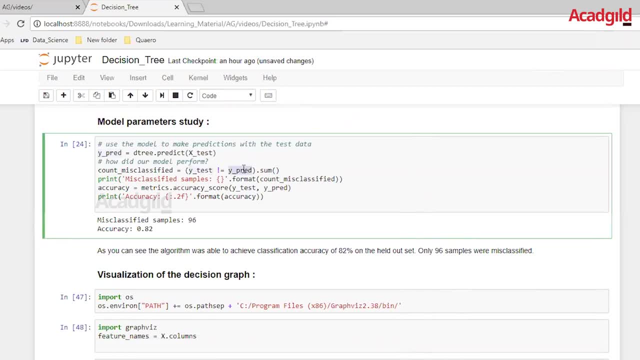 Now the results will be the result of the Y test and Y pred. The current problem which you are solving is a classification problem, So we can directly compare the results between the Y test and Y pred wherever these two values are not equal, and then we can take their sum. This will give us the 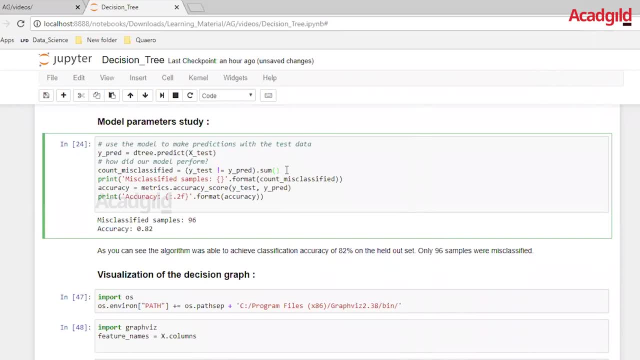 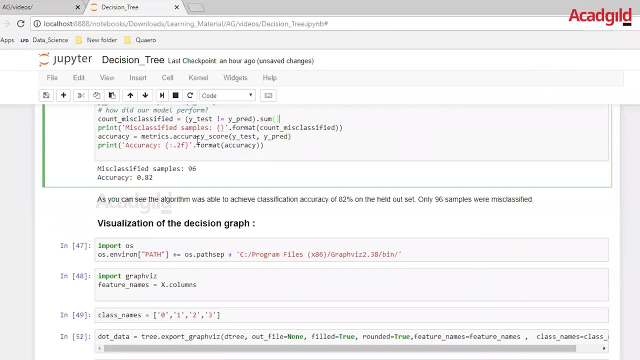 count of the total mis-classified samples which are present in the final predictions done by the dysentery which we have trained on the 70% of the train dataset. The next thing you want to print is an accuracy score. The accuracy score will do a comparison between, again, the ytest and ypred and it will 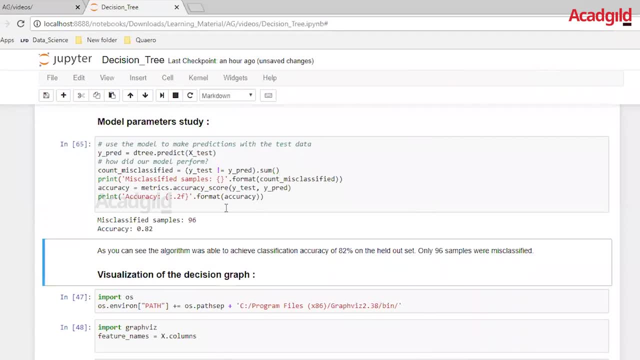 give us the final accuracy. So let's execute this command and then see what are the results. So we can see that the misclassified samples have a total count of 96 and corresponding to which we are getting the accuracy of 82%. Let's go. 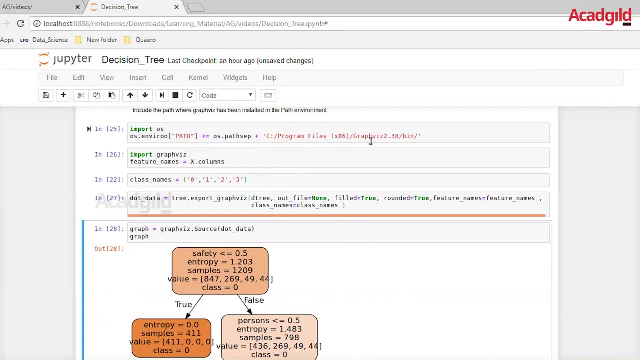 with the visualization of the dysentry which we have made earlier. Before I proceed with the actual implementation part for the visualization, please make sure that you have installed the graphvis library. Also, if you're on Windows platform, make sure that you have installed the graphvis software from. 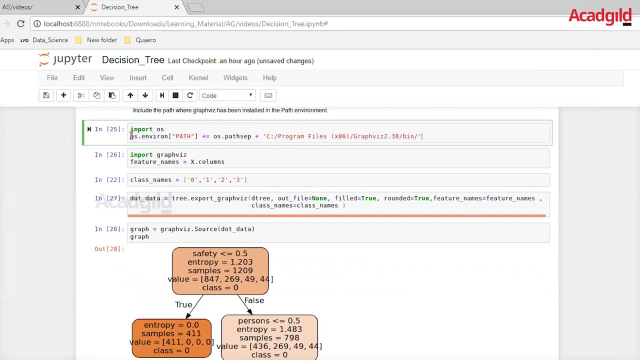 the given link. If, in case, you have missed to add the path variable for it, make sure that the same thing is done right up over here, only by importing the OS module. Let's execute this. The next thing is to make sure that we are having 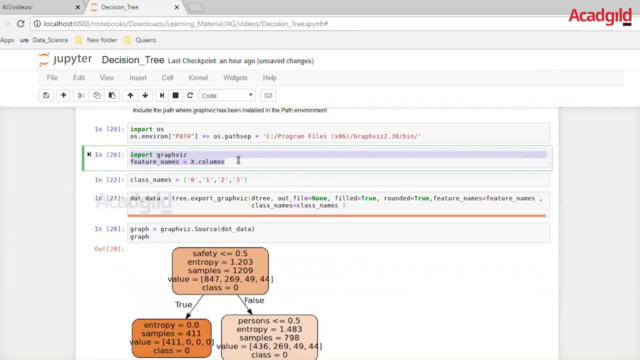 the feature names which are coming from directly the initial data set, which is the x, so it will have all the columns. The next thing is to make sure that the class names are represented as a strings and not as the integers directly. Let's call the exportGraphvis function, which takes into account the dysentry. 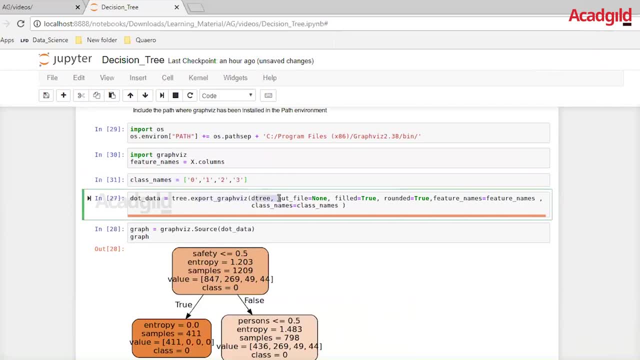 which we have built, and also the feature names, which are the column names of the dataset, and the class names, which are the final labels of the dataset. If you want, then you can make use of the out file option as well, which will create a dot file instead. 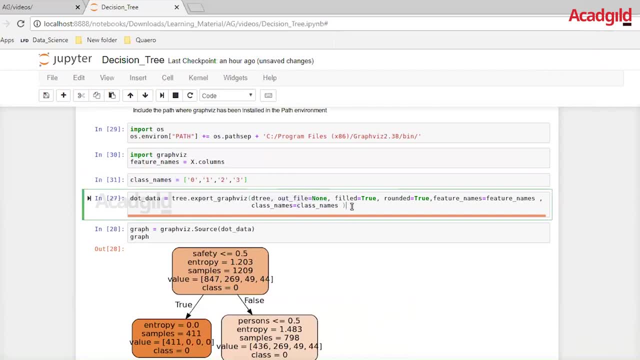 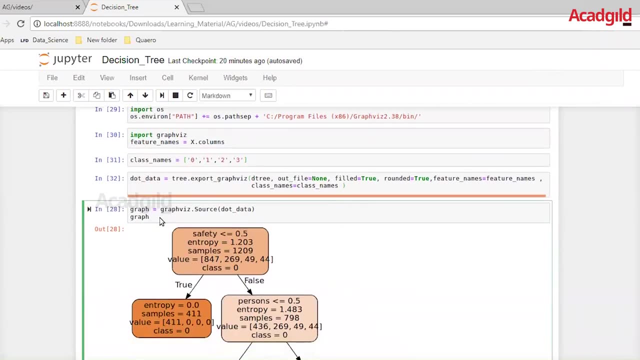 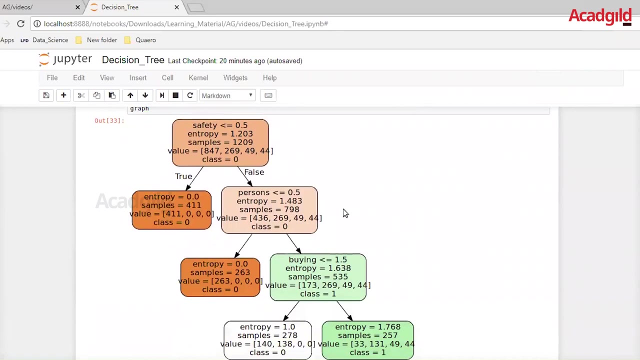 and it will store in your current working directory. Let's execute this. Now we have the final graph and we can visualize it. So this is the final graph which we have of the above tree, which we have created using the decent tree classifier from the scikit-learn library. Let's try to understand what exactly the 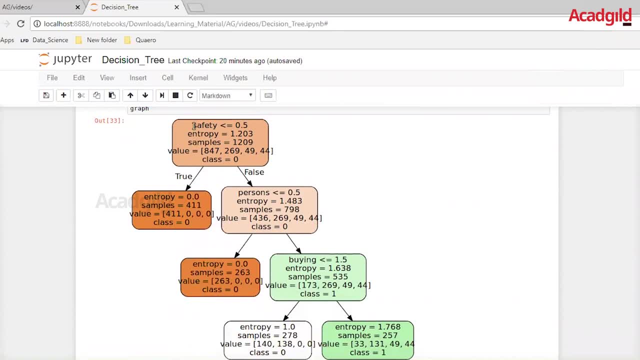 output is about. So, if you see, the first step is about the root node, which has the values of the four different classes. Also, the split on this root node has been made using the safety column, which is if the value is like less than 0.55, and if it is true, then it will go on its left side If it is greater than 0.5.